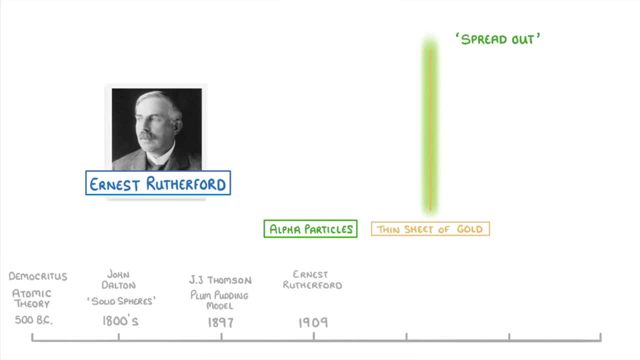 be strong enough to affect them. Weirdly, though, what actually happened was that some of the alpha particles were deflected to the side, and a small number were even deflected back the way they had come, And that's because the weak spread out positive charge wouldn't be strong enough to affect. 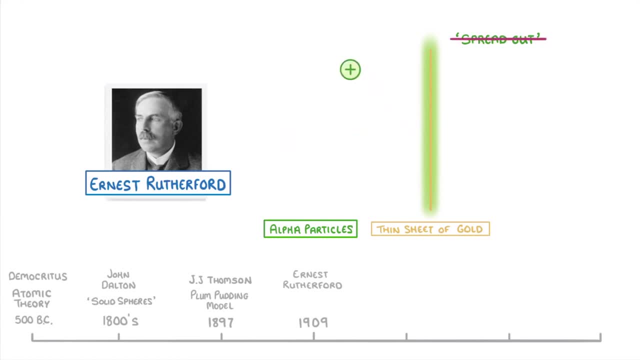 them, And that's because the weak spread out positive charge wouldn't be strong enough to affect them, Proving JJ's theory wrong. Because of these results, Rutherford suggested his nuclear model, which proposed that instead of a general field of positive charge, there were some sort of compact nucleus which contained 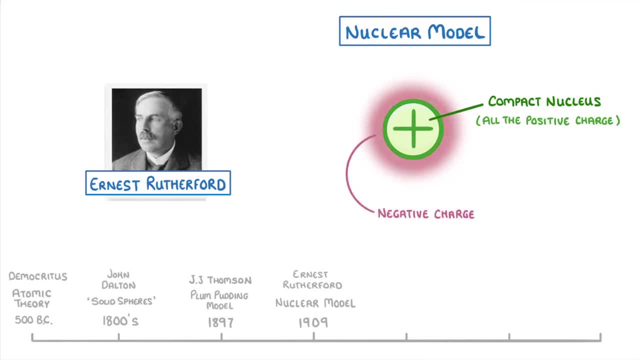 all of the positive charge of the atom, And he thought that the negative charge must exist in some sort of cloud around this central nucleus. At this point, Rutherford was already pretty close to how he currently understands the structure of the atom. But his model had one important flaw, namely there didn't seem to be anything stopping. 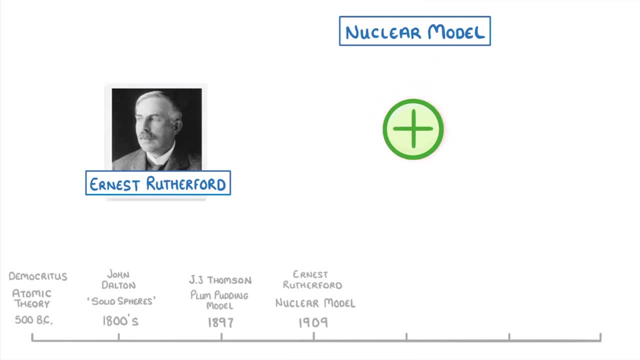 this cloud of negative electrons from rushing in towards the positive nucleus, meaning that the atom should just automatically collapse, which we know it doesn't. Just four years later, though, in 1913, a man called Niels Bohr suggested a solution. He 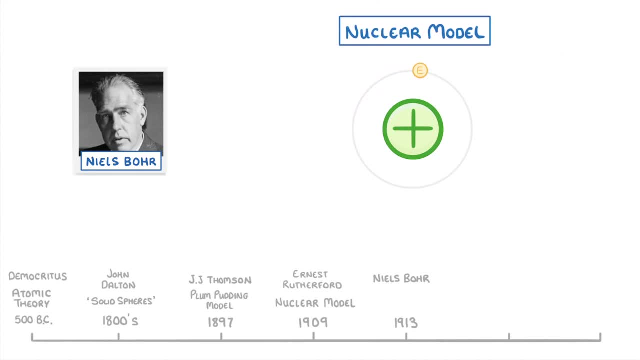 suggested that the electrons all collapse automatically, And that's when he found out that the electrons orbited the nucleus in a similar way to how the planets orbit the sun, And also that they were held in shells. This idea was really important, because the orbiting of the electrons is what prevents 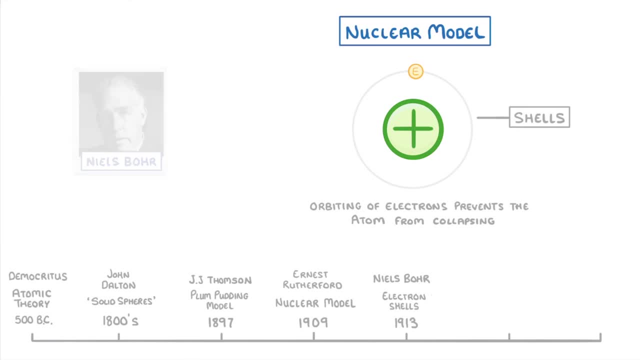 the atom from collapsing. In the years since then, many experiments have supported this model, and it's pretty much the same one as we follow today, with just a few small changes. Further experiments by Rutherford found that the positive charge in the nucleus is actually made up of small, discrete particles, which 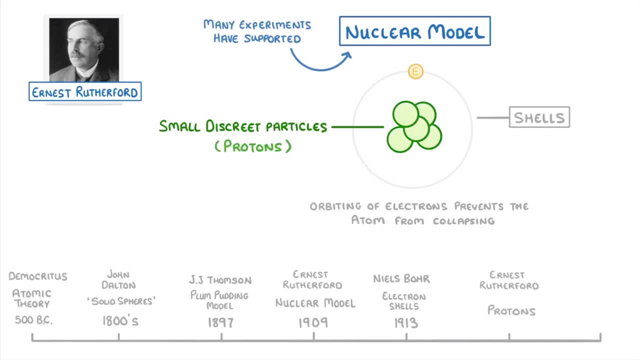 we now know as protons, And a short while later, a guy called James Chadwick provided evidence for neutral particles in the nucleus, which we now call neutrons, And that's pretty much how we understand the atom today. Anyway, that's everything for this video, so hope that was useful and we'll see you. next time.